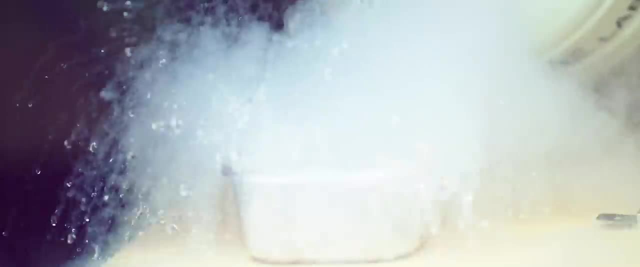 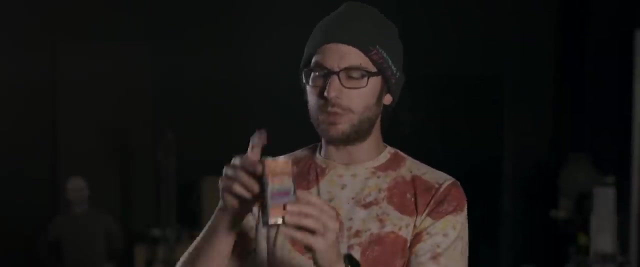 But we are here to levitate an object. so what does liquid nitrogen have to do with magnetic levitation? Because you can make magnets levitate without it right now, And to demonstrate this, I'm going to use Inks, Levitating Rings, which is a fun product that Michael Kevin and I made for the Curiosity Box. 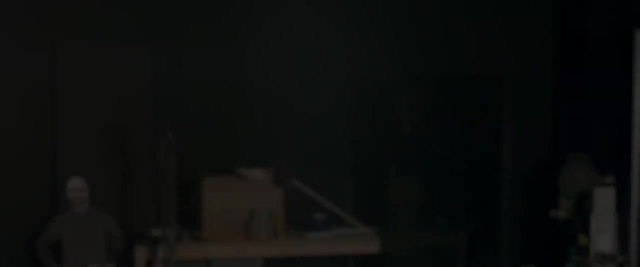 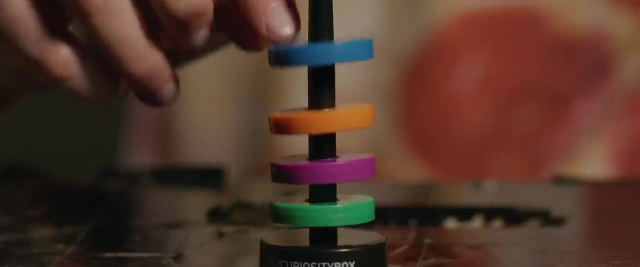 There's a link down there in the store if you want to get your own, Or you can use any two magnets that you have at home. Now let me show you how this works. If these two magnets have like poles facing each other, they repel each other. 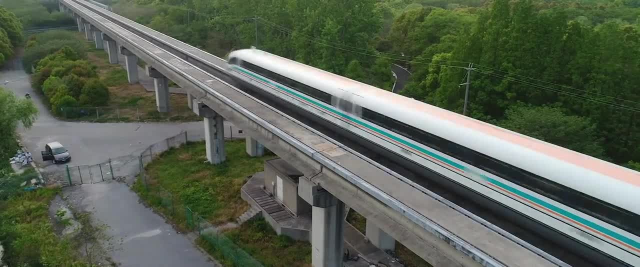 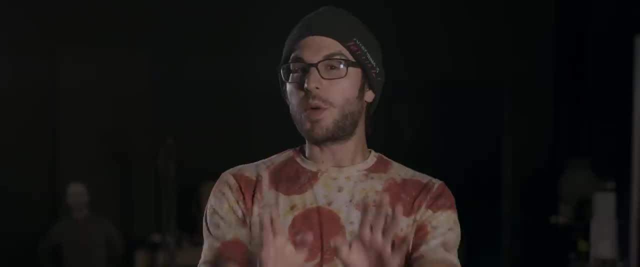 It is the same principle. It's the same principle for how maglev trains work, And the opposite occurs if we flip the magnets around. They're attracted to each other. But what we're doing here is not regular magnetic levitation or maglev. It's superconducting maglev which is different. First of all, let's discuss superconductors. A superconductor is a material that exhibits two incredible properties when it is cooled below a so-called critical temperature. The first is that they have zero electrical resistance. 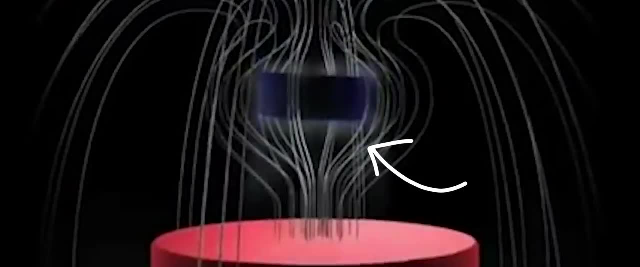 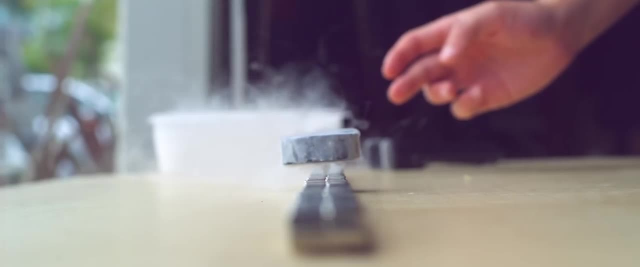 The more important for our purposes is the Meissner effect, which causes a superconductor to completely expel magnetic fields when they enter their superconducting state. What that means is that a superconducting material will actually levitate over a magnet. 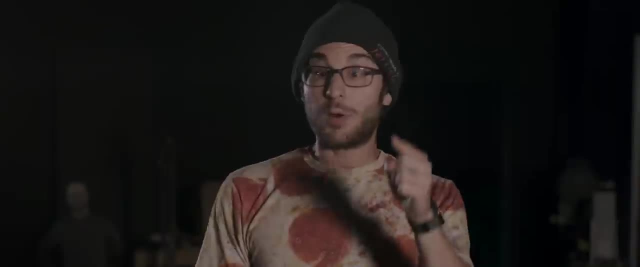 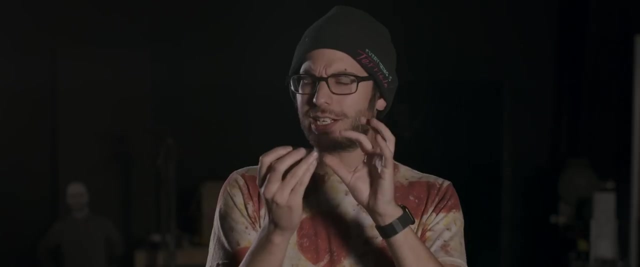 even though the material itself is not magnetic. Now, this is our superconductor, a small disk made of yttrium, barium, copper oxide. Actually, in this whole thing, the superconducting material is just a tiny sliver of crystal. 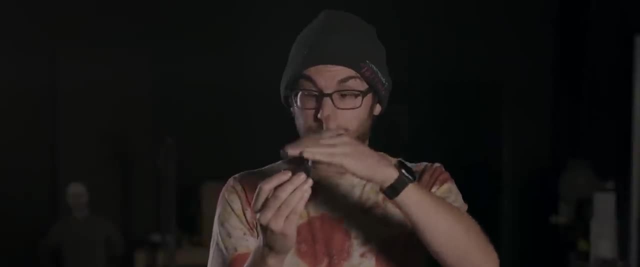 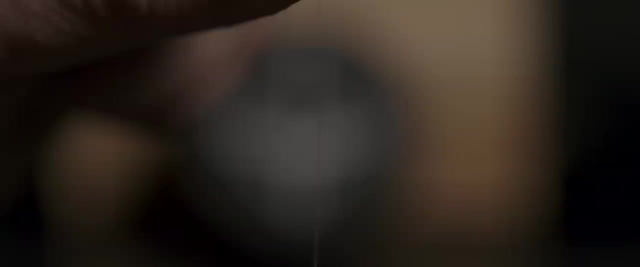 grown on top of a stainless steel core and covered by a protective layer of silver and aluminum. And when I say a tiny sliver, it really is. It's just three microns thick- 30 times smaller than the thickness of a human hair. 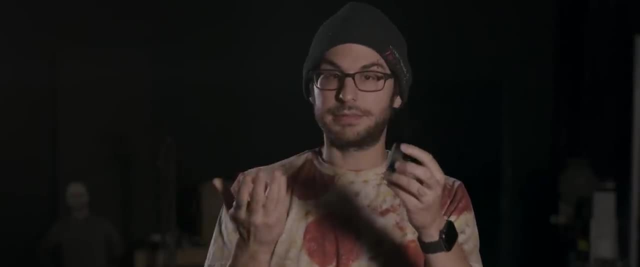 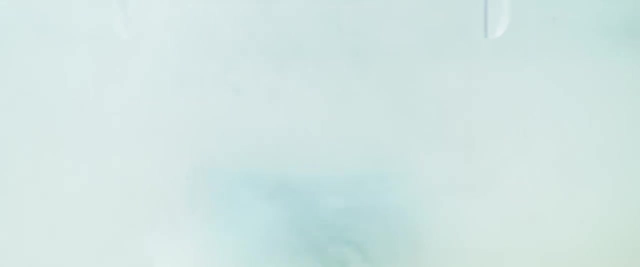 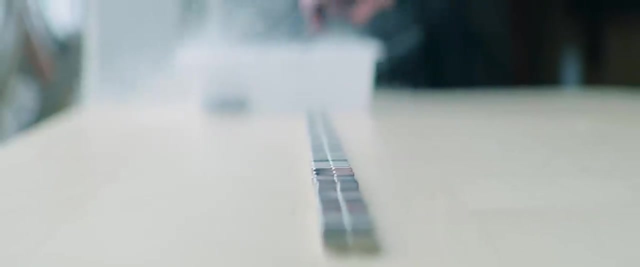 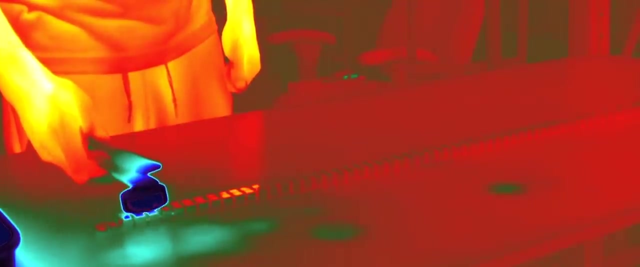 And if I were to put a magnet next to it? well, nothing happens, because it will only levitate when it's below that critical temperature, which is why I drowned it in liquid nitrogen. One of the most amazing things about superconducting levitation is what you see here. 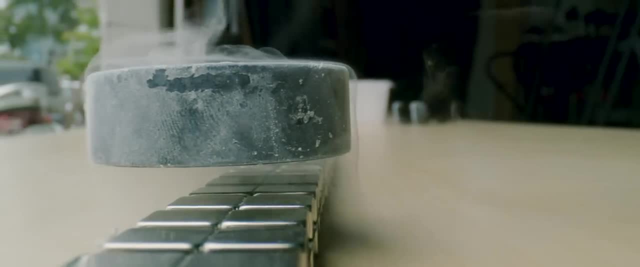 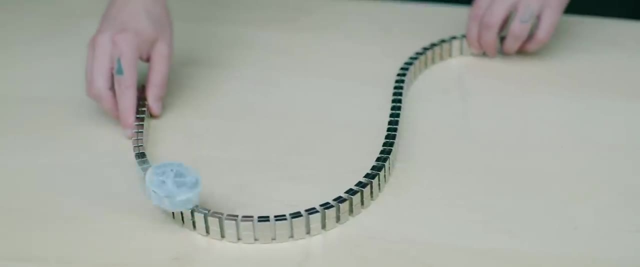 Not only does the disk hover above the track, but it can hover below it as well. In fact, we can shape the track any way we want, and the disk zooms along at exactly the same height, no matter its orientation, with no friction or resistance.